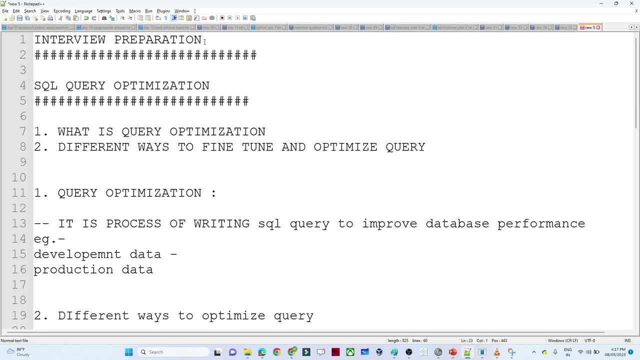 hello everyone. so we will continue over the interview preparation part. in the previous video we have seen couple of the question which was generally asked in interview, so we will continue with that and in this particular video we are going to understand and most important topic, that is, a sql query optimization from an interview perspective also and from a development perspective. 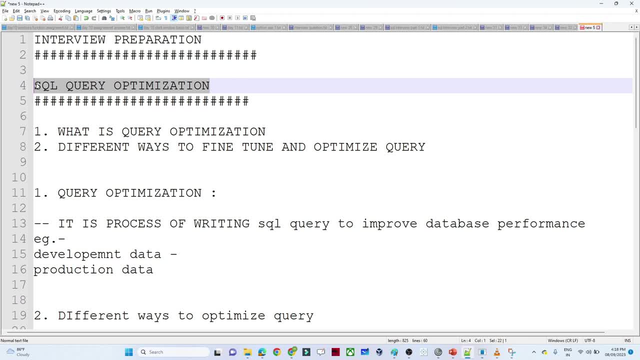 also, all the developers should know what are the different optimization technique whenever we write a query, how actually we can write in an efficient way. these are the things actually everyone should know. okay, so that actually we are going to discuss, so we will start with the what is a query? 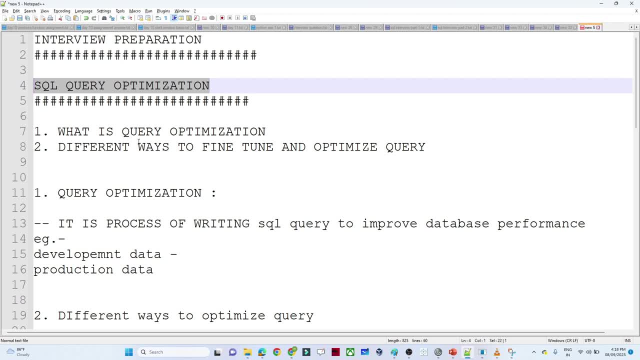 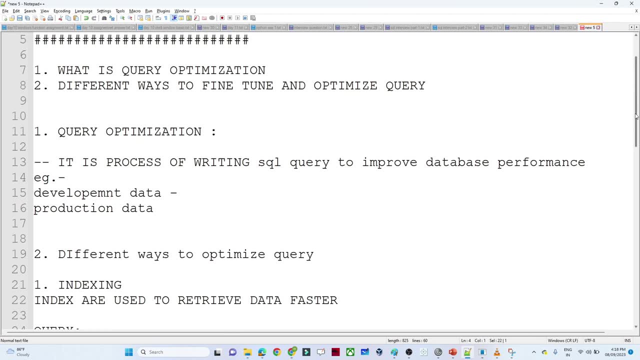 optimization. first we will try to understand what is query optimization and then we will see what are the different ways through which actually we can optimize our query. okay, so let us start with that. the first one is like query optimization. okay, what is query optimization? so it is a process of 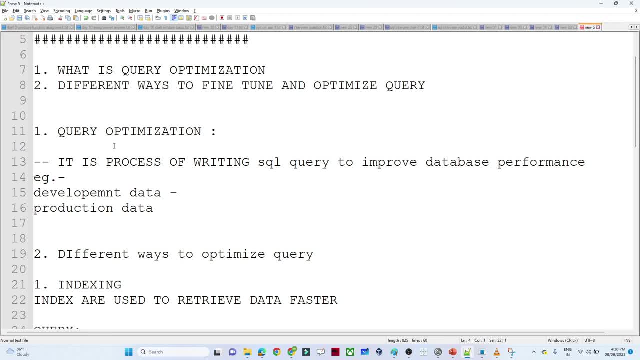 writing a sql query in a efficient way to increase the database performance. okay, so for taking example, suppose you are working in a development industry environment. suppose you have written a complex query. even though you are executing those query, you are not seeing any performance issue because, generally, what happened whenever we work in a 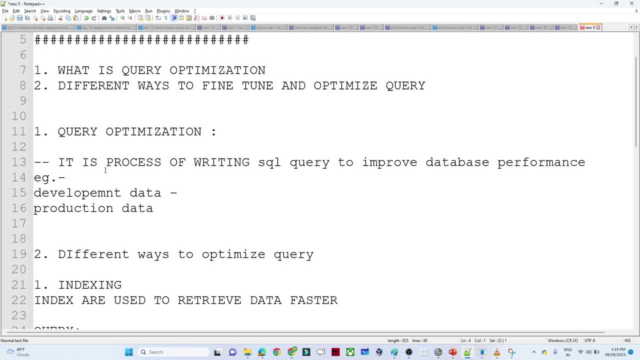 development environment, we generally will be having a less data. okay, and the same thing actually when you are testing into the production environment, right there, actually we generally get millions of the records and more than that, right, so in that case the performance issue comes into the picture. okay, means our your query is taking a longer time. 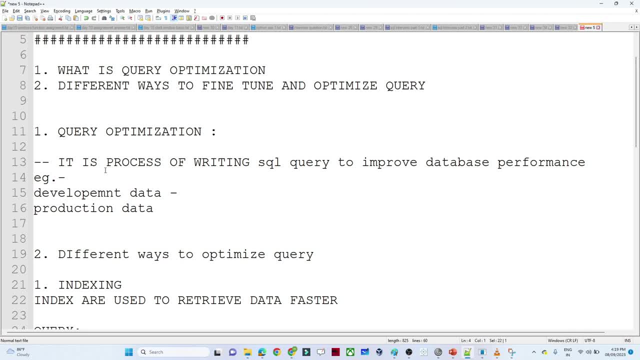 it is not increasing the user experience. so there are so many kind of the issue we generally face. okay, to overcome this, we can use a- we should know the query optimization technique. okay, now let us try to understand how, what are the different ways through which actually we can optimize our query? 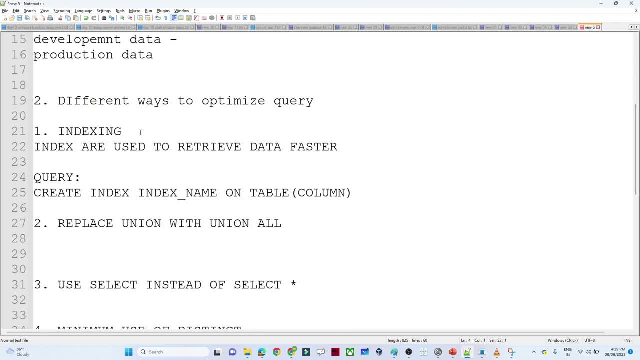 okay, so first is indexing. what is the first? first one is the indexing. okay, what is indexing? index are generally used to retrieve your data faster. okay, when we use a indexing right, it actually helps to retrieve our data faster as compared to the not using an indexing. okay, 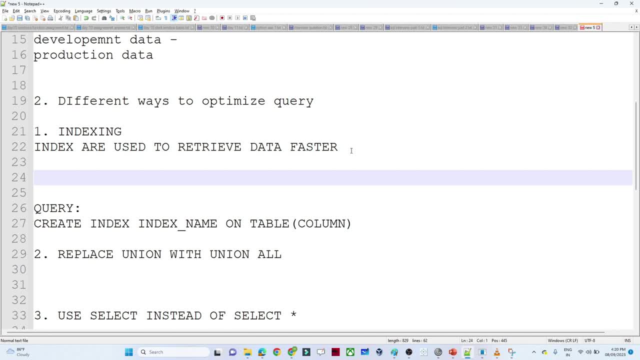 for taking example, suppose you have a table. okay, suppose you have a table. in this table you have a millions of the record, you have a millions of the record. suppose, uh, millions of the records is there in this particular table. okay, now, what actually you are searching in this particular table? you 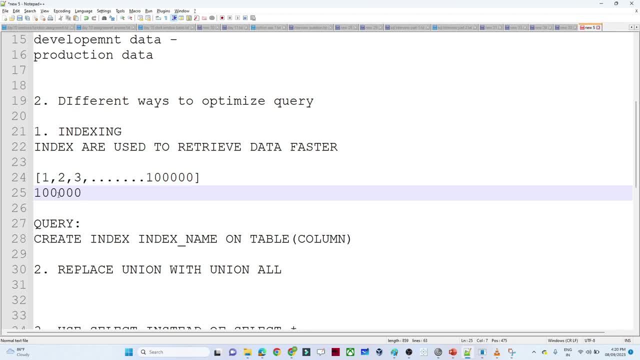 are searching a 1 million record. okay, suppose you are searching where salary equals to the 1 lakhs. okay, here actually what you are searching. you are searching on 1 lakhs- okay, give me the result- where salary equal to the 1 lakhs and you have a this much salary. okay, this much record also and this much salary. 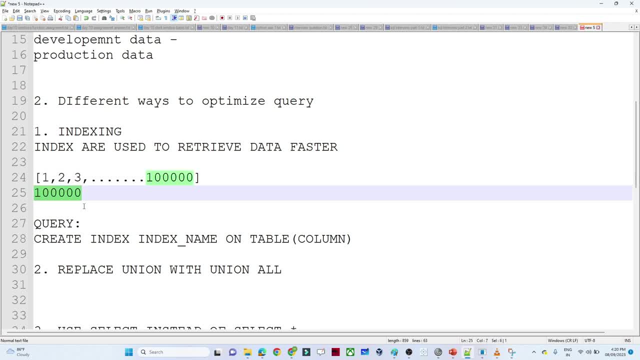 record also you have. okay, i am just taking example. okay, now when you write a query right, where, so what actually it will happen? it will try to search into the whole table. okay, and it is present in the last right. you are searching in the whole table. where suppose you have a 1 million? 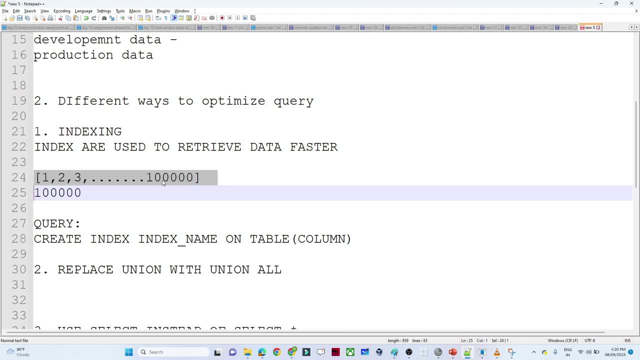 record. so you are searching in the whole 1 million record that increase the performance issue. okay, to other stream, set g, kick spread and you see the success rate. so thisафi is given these three staples because the going to focus on as a strategies, using this, how the problem is. 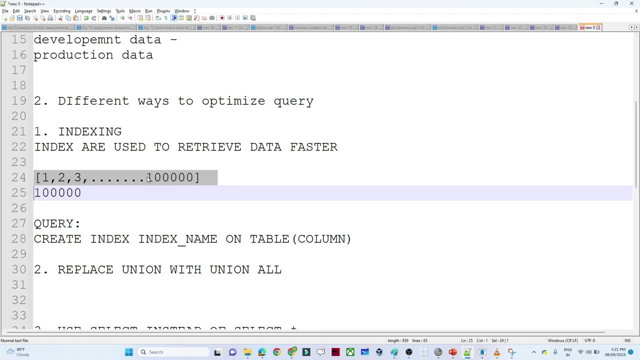 parallel engineering deal will takes place from. you know what i am generalizing how your, and then we will see in詩. do we have an indexing? do we have a triple identity or a common system? um, so what we are talking about here are the other technologies and information. 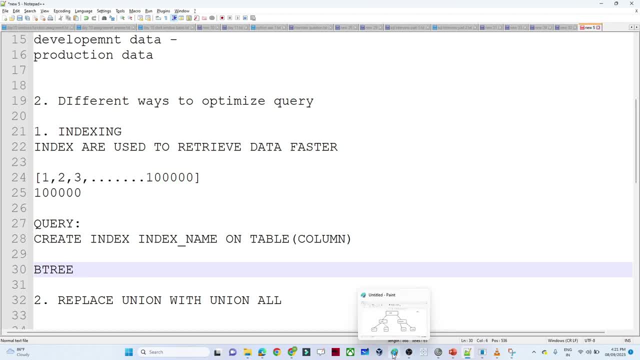 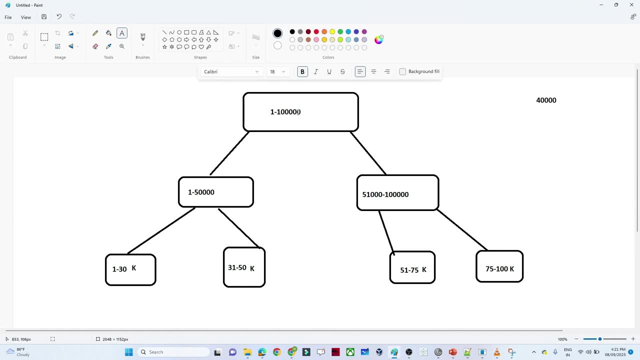 and also increase the performance. okay for taking example. okay, suppose this is a my table. okay, or you can take an example of the employee id. suppose you have one to one million employee id. now you are searching the employee id equal to the 40 000. okay, now what you will do when you will use a. 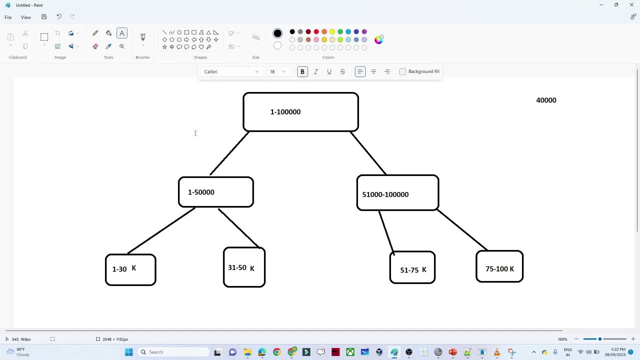 when you will not use an index, it will do a full scan into the whole table. but when you are using a indexing, right, it will use a b3. okay, so how? actually it will search. you are searching for the 40 000, right? so first it will come into this particular, the first graph. okay, one to one million. 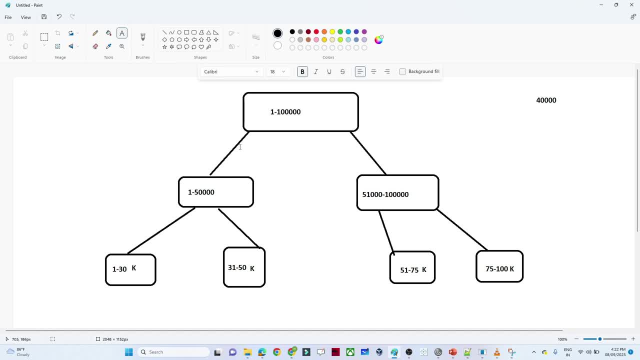 okay, now we are searching for the forty thousand. okay, then it will directly go to the left node. it will not go to the right node because forty thousand is will be present here, right? it will not go to the right side because, right side, we have information from the 51 000 to the 1 million. 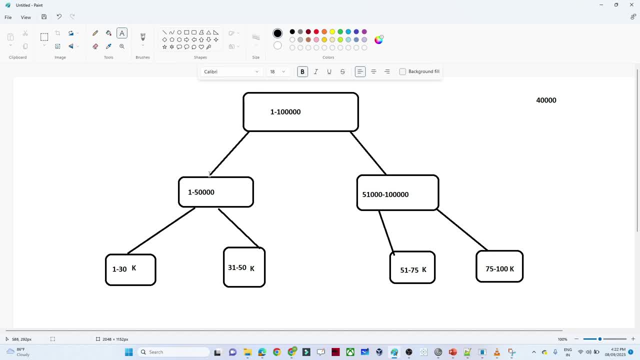 so in that bucket it will not go. it will search into the left bucket. okay, once it will come into the left bucket, okay, now again whether we have a record into the 50th one to fifty thousand right. so again it will search in the left side. you can see we have one to thirty k in the right. 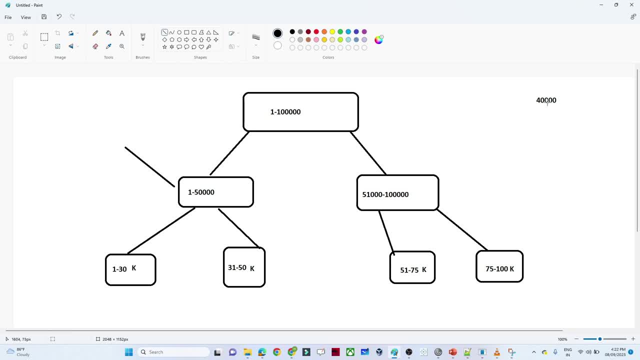 side, we have a thirty one to the fifty k. okay, what we are searching? we are searching for the forty thousand, so it will directly go to the right side. okay, so this is how the b3 structure works and it will improve the performance. okay, i have just given you the high level idea, but that is how. 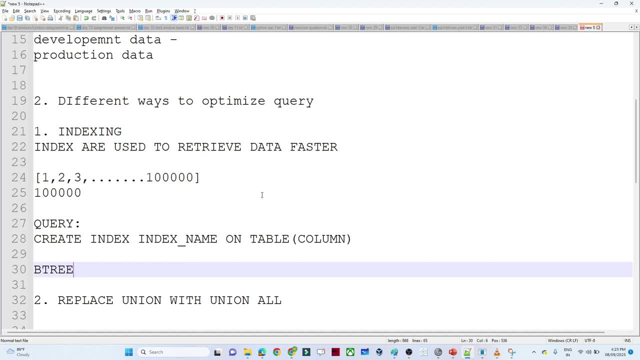 actually it works. i hope you got it okay. so this is how actually it was and it actually tried to improve the performance. so always try to use the indexing, which generally help you to increase the performance. okay, if you want to know more about it, please do comment so that i will make it. 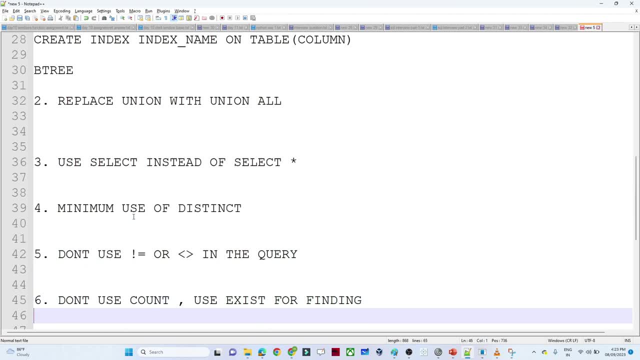 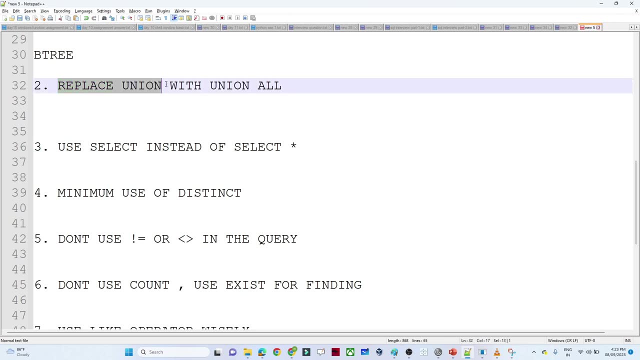 separate videos for the indexing. okay, now let us try to understand the second method. what are the different other method through which actually we can optimize our query? the second is the replace union with a union- all okay, replace union with a union- all. so what generally happen when we use a? 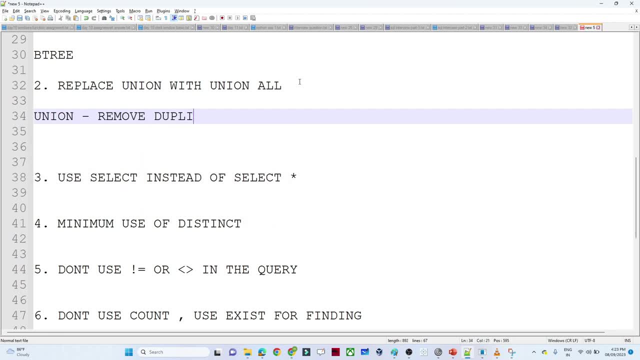 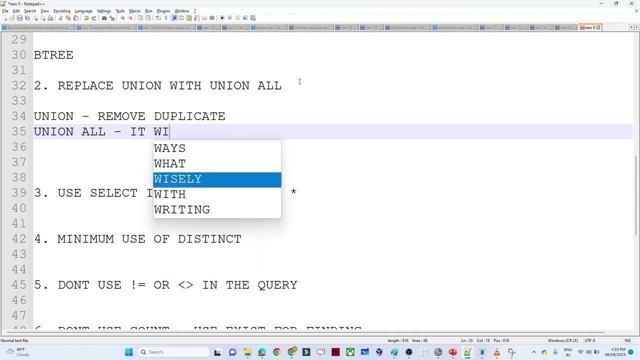 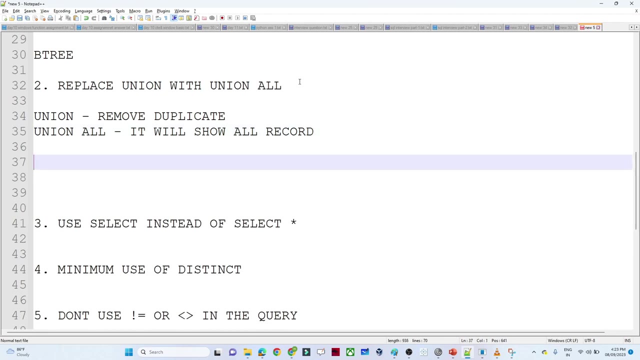 union, right, it will remove the duplicate. it will remove the duplicate and this is a time consuming. it is a time consuming also, and when we use a union, all it will show all record. it will show all the record record, even though duplicates is or there or not. okay means when you aware, like in the table, you don't have any duplicates. 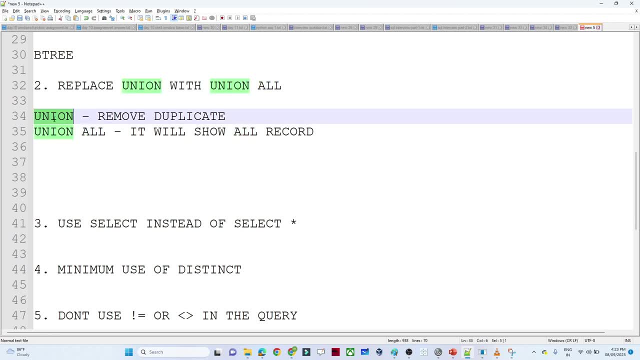 avoid using the union. all. avoid using the union. use a union all okay, because whenever you have to use a union or the union, all right. always try to use a union all because it will. it is a efficient as compared to the union because, in the case of the union, right, it will first remove the 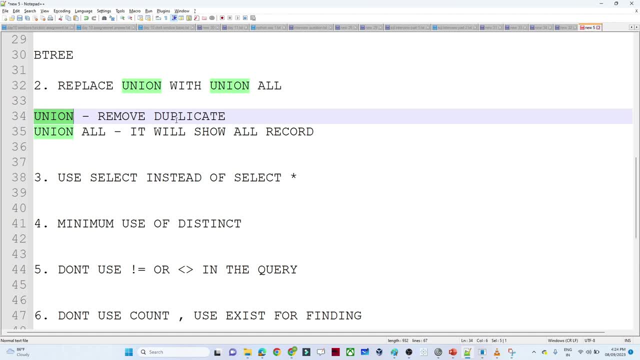 duplicates or the data. so it is a time consuming, okay. so that is why avoid using the union. use a union, all okay. now, third one is like select instead. you select instead of the select star. so generally, what happen when you join organization? you get a database and you try to search a table, okay, when 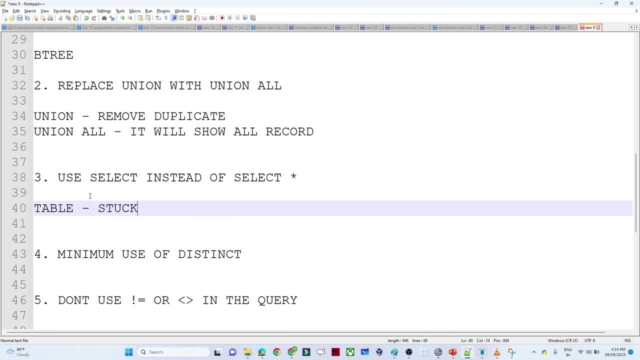 you are searching a table, generally, what actually happen? it generally try to stuck also, or sometime it get lock also or it, or it is taking a longer time. this kind of the issue generally we face okay, because what we do we try to use a select star from a table. this kind of the query we try to write: okay, that is not a efficient. 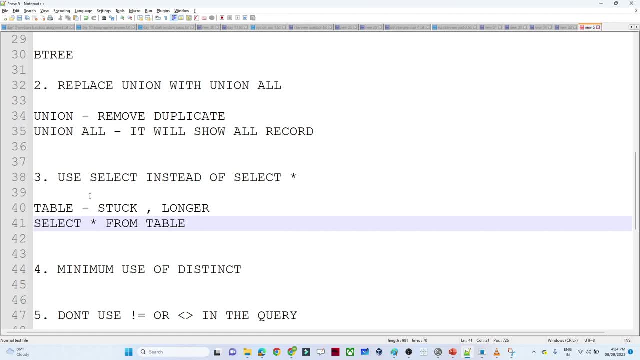 way, because this will try to search the whole table- okay, and this is a time consuming also, and it will it take the resources also, okay. so instead of that, try to use a select column name. okay, column name from a table: okay, whatever the column you are interested, you can use that, or you can use: 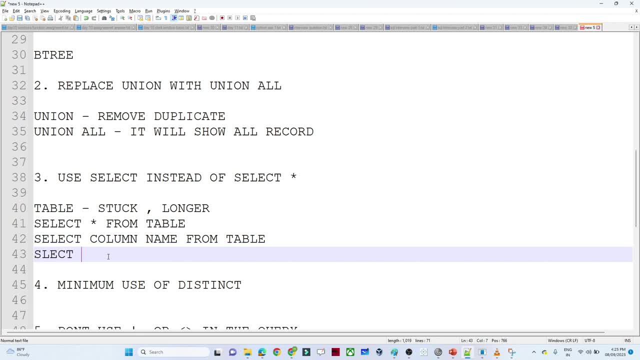 a limit limit also you can use, like you can use a select of five from a table, okay. or you can use a select star- select star from table limit table, a limit five or something okay. so this kind of the thing actually you can use so wide using a selector, you can use a limit, okay. and 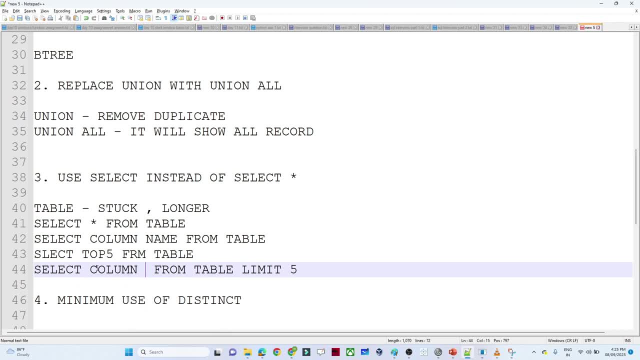 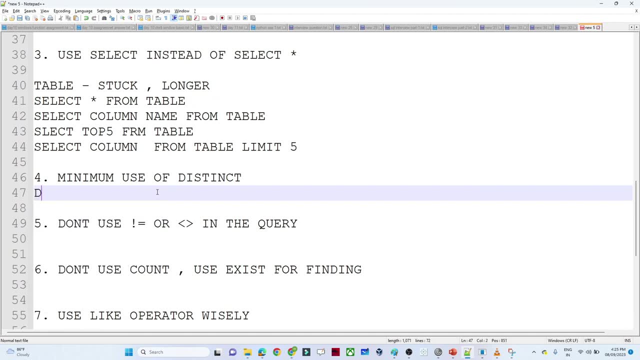 here also, you can, if you know the column, and try to use a column. okay, that is the efficient way, okay. the next thing is like minimum use of distinct. okay, because in the case of the distinct right, what does distinct do? it will try to give you the unique record, it will try to give you the unique. 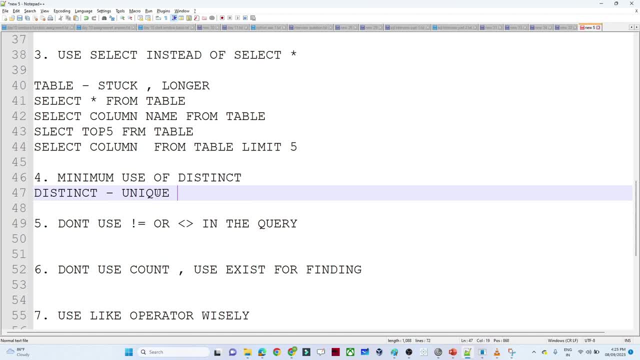 record, in this case the. all the duplicate removal happens right, so it is time consuming, so try to avoid using the distinct okay. now the next thing is like: don't use is not equal to the okay, so suppose you have to some condition you are putting where you want to check. the is not equal to the. 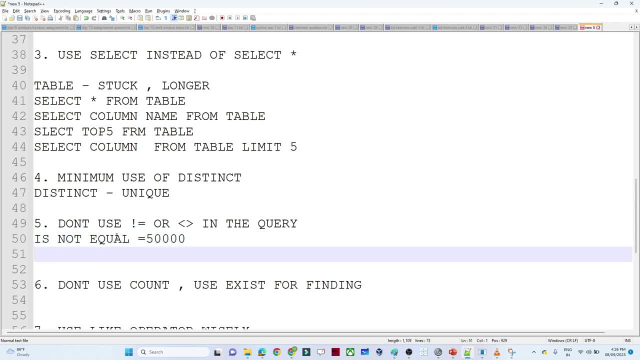 is not equal to the 50 000. this is the condition you want to check. okay, so if in this kind of the case, if you have some other, try to use that, because when you are applying a indexing and when you are using this is not equal. 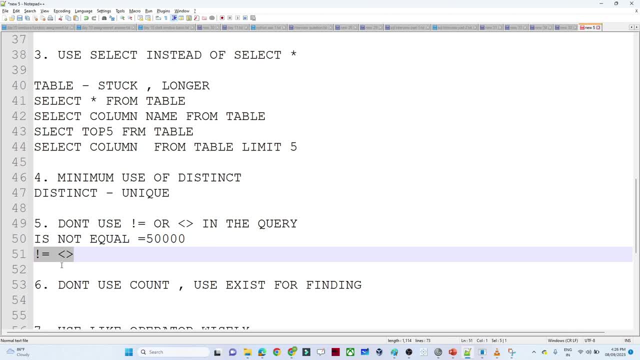 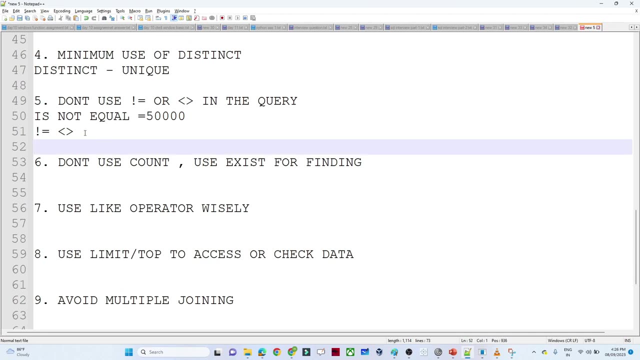 to: okay. in this case, the indexing doesn't work. okay, so don't use is not equal. that is the one efficient way and try to use some other method. okay, or you can use a joining, also, you can prefer it, okay. okay, so, if you can achieve the same result, okay. so that is the thing you have to remember, okay. 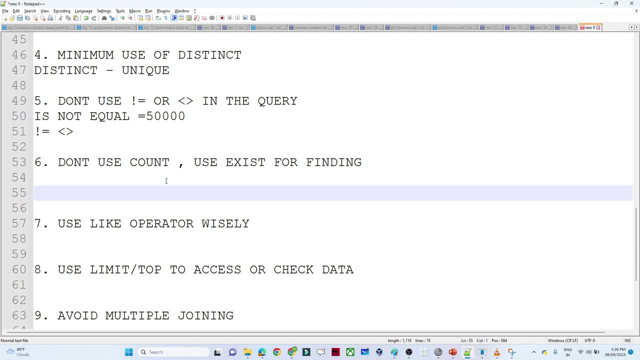 don't use count. use exist for the finding. suppose you have to find a result in the table where the monies is present or not? okay, where employer name is equal to the monies is present in the table or not, okay. so instead of writing a query like select count from table where uh name equal to 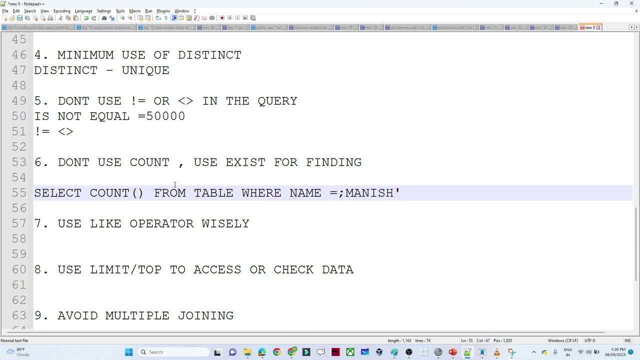 the monies. okay, instead of writing this, try to use a. try to use a exist. try to use a exist because when you use a exist, right, what generally happen? suppose you have one millions of the record. okay, in the one millions of record, if any of the record, it is matching with the existing condition in the 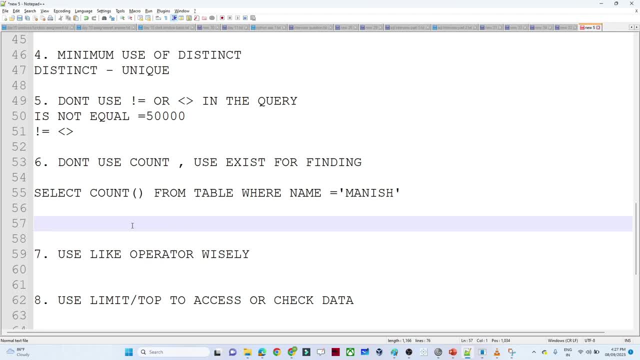 that in that case only, it will get stopped. suppose it is matching in the second record itself, so it will stop it and it will give you the results. so that is how the exist works. okay, so try to use exist instead of the counts. that is the thing you have to remember. okay, the next thing is like use. 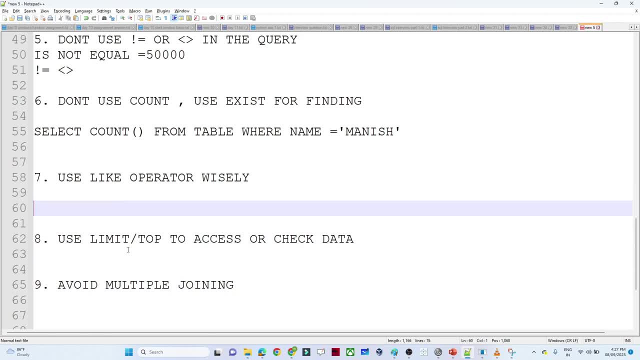 like operator, wisely. okay, so suppose generally, what happens? suppose you have to search all the employee details. who is starting with the name av, av. okay, so, instead of writing this, instead of writing like this condition, okay because you have to write like this condition, okay because you have. 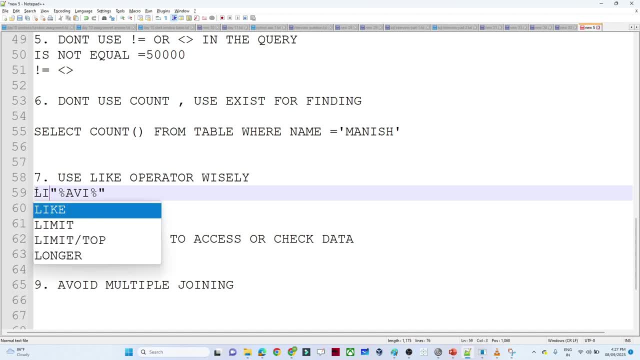 to write like this condition: okay, because if you write where name equal, where name like percentage, av, percentage, okay, in this case, what actually happened? it will try to scan the whole table instead of that. what actually you can write, you can write av. it is starting with the av right. 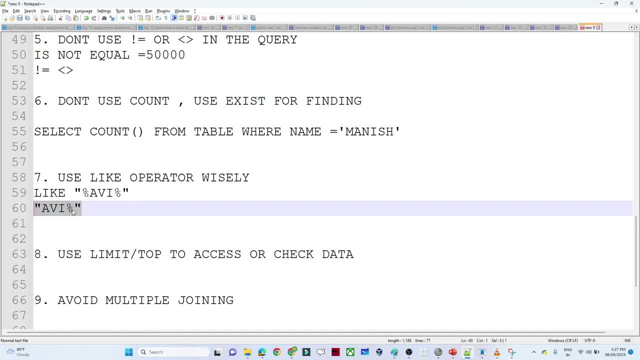 okay. so this is the thing actually we have to remember, okay, we have to use like operator wisely also okay. and the next one is like use limit order top that actually already we have seen. okay, suppose you want to see only the how the table structure looks like. so always, 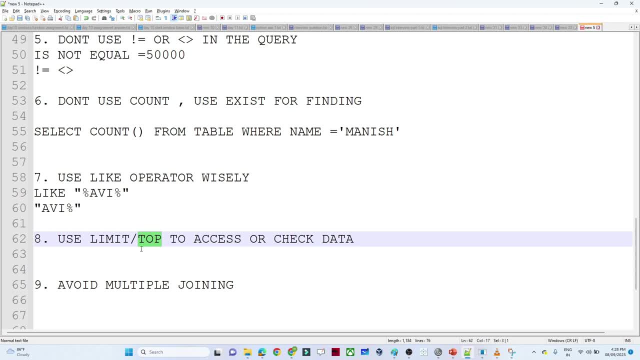 try to use a limit top instead of using the select star from the table, okay. and the next thing is like avoid multiple joining. we all know like the joining takes a huge time, okay. so if you are using a multiple joining, try to minimize that. try to use some term table and, based on that, actually try to 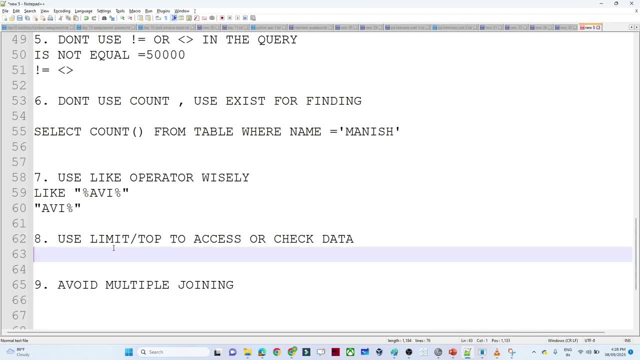 try to use that, to utilize that, so this kind of the thing which we have to remember, okay. so these are the different ways which, through which actually we can optimize and which we should aware, okay.